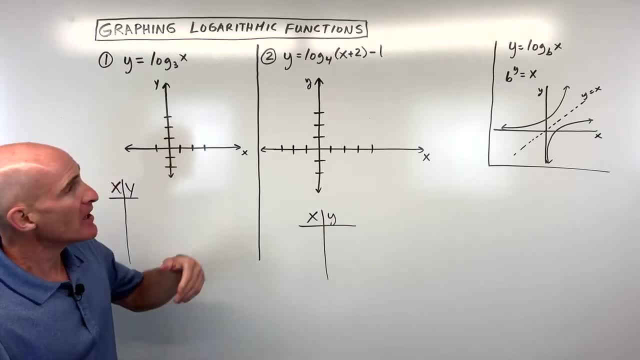 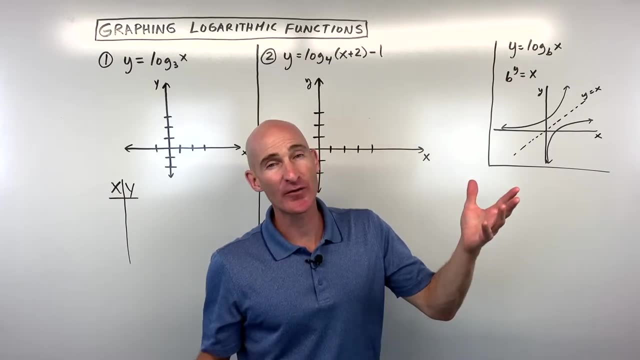 showing you. So let's dive in and I'll show you how this works. So the first thing we want to talk about is when we graph a logarithmic function. we want to understand that logs and exponential functions- they're inverses of each other, and you previously learned how to graph exponential. 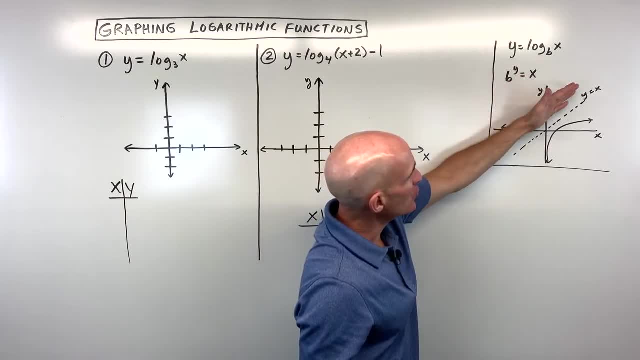 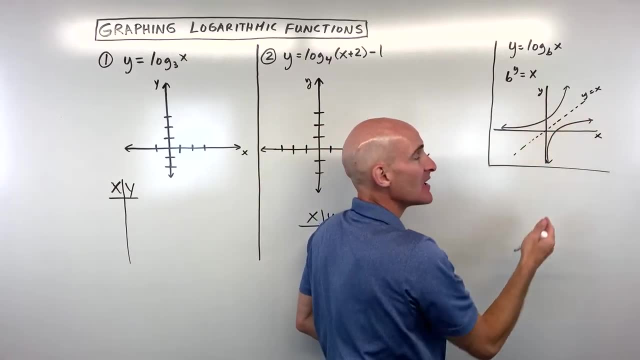 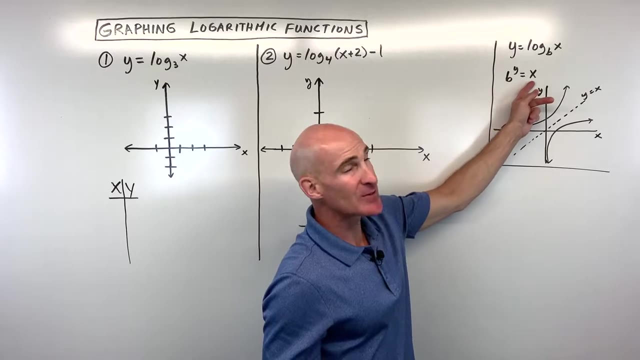 functions and when you find the inverse is what you do graphically is you reflect it over this line. y equals x, So when you reflect it, you're going to get a graph that looks something like this: This is a logarithmic graph, So what you can do is you can rewrite the log into exponential. 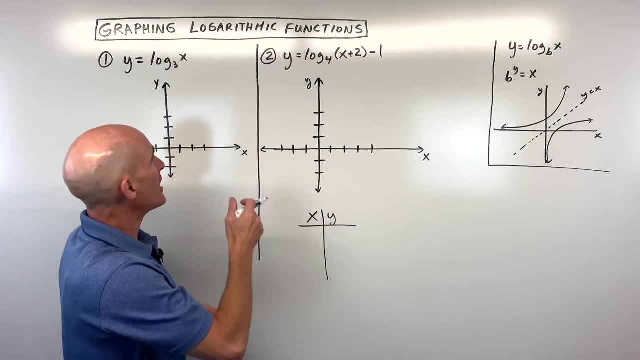 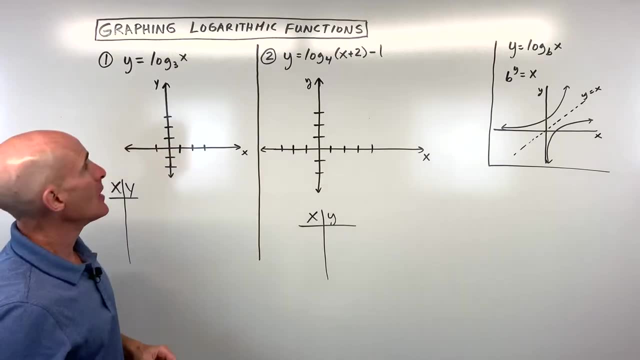 form, and I'll show you how to do that in some of these problems. So let's talk about example number one here, where we have: y equals log base three of x. So how do we graph that? Well, you can do that by using the equation: y equals log base three of x. So how do we graph that Well? 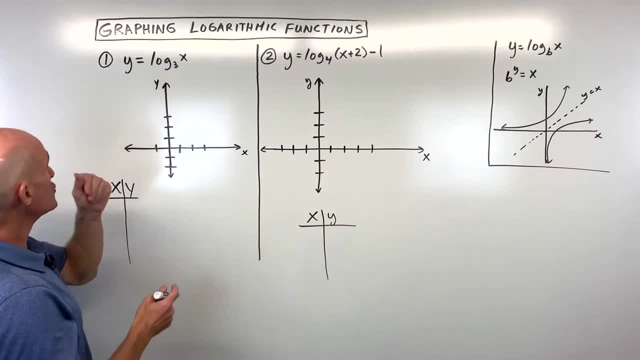 you can do that by using the equation: y equals log base three of x. So how do we graph that? Well, how we said that logs and exponential functions are inverses. So what you can do is you can exponentiate or raise both sides using this base three. So if these bases match, 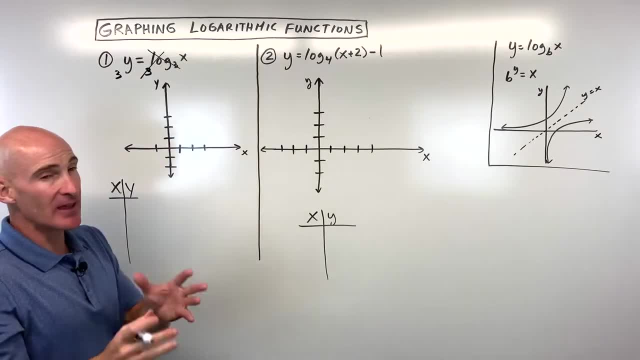 the exponential function and the logarithmic functions. they undo each other. So now what we have is we have this equation: x equals three to the y power. So we'll make a table and we'll plug in some values for y, not x, but y, So negative, one zero and one, So three to the negative one. 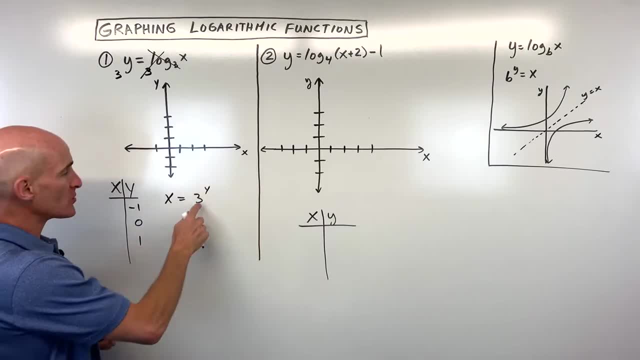 when you have a negative exponent you take the reciprocal. So three to the negative, one is going to be one third. Three to the zero, anything to the zero power is one, and then three to the first is three. So now if we plot these points, let's see we've got right: one third down, one, one zero. so 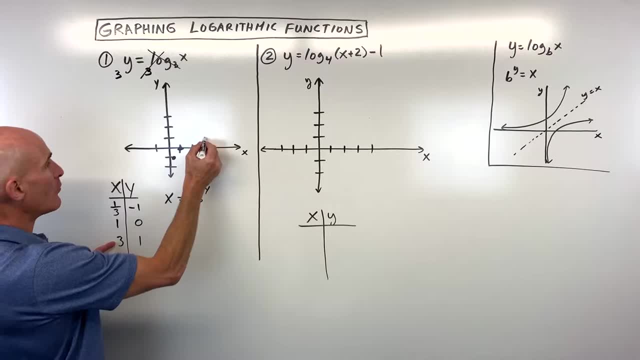 that's right, one up zero. and then right, three up one. And here's your logarithmic graph. right there. Now, when you want to find the domain, what you want to remember is that you can't take the log of zero or a negative number, So whatever is here you can. you can basically say: x equals zero and 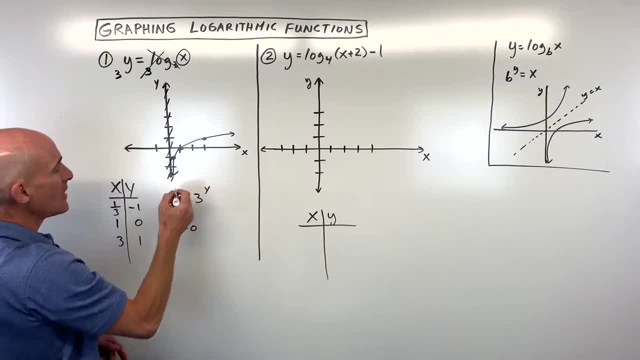 that'll give you this vertical line which is right here on the y-axis. Okay, and if you want to find the domain, this quantity here has to be greater than zero, because it can't be zero, can't be negative. So that'll be your domain: everything greater than zero. or if in your, if you're in, 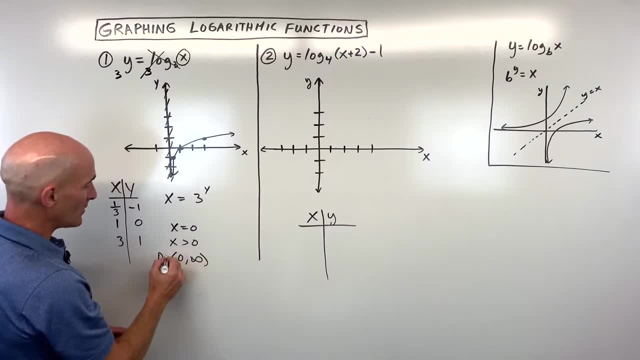 pre-calculus, you could write this as zero to infinity as your domain, Okay, and then notice that this graph goes down and gradually up, up, up, so the range is going to be all real numbers. or if you're in pre-calculus and you're learning the interval notation, you could say negative infinity. 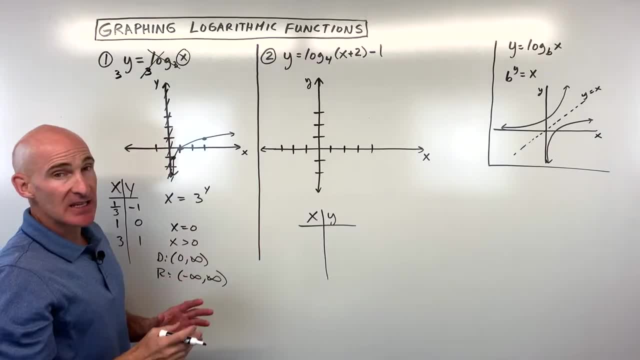 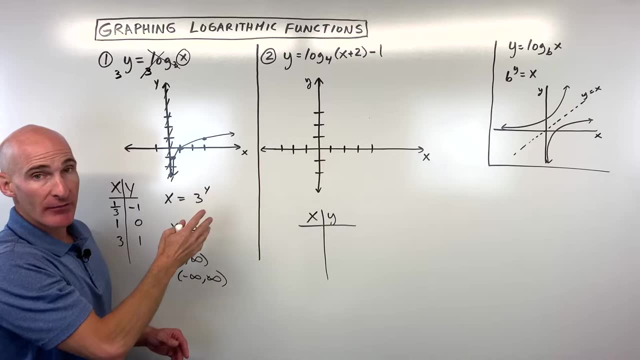 to positive infinity. So that's the basic idea is basically rewriting this into the exponential form and then you can make a table and graph. Let's look at a little bit more complicated problem now where there's some transfer. So if we go over here to example number two I mentioned, there's a couple different methods to 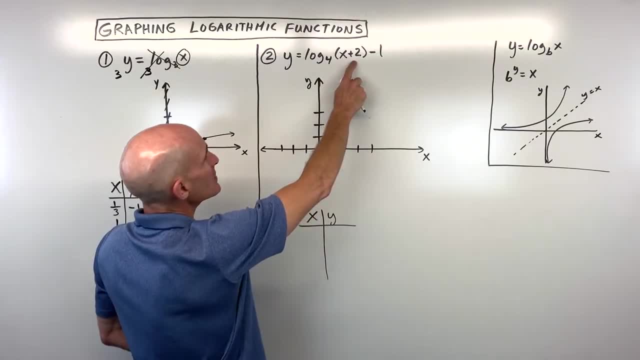 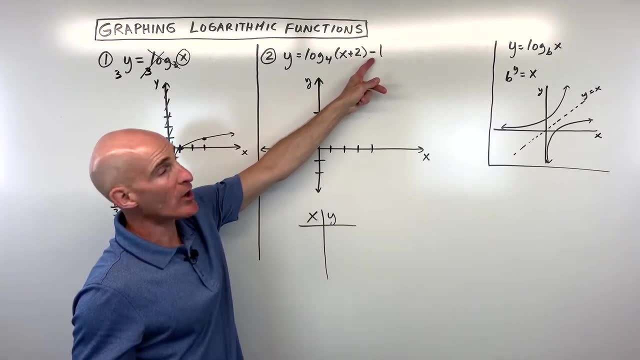 use here. The first method we're going to talk about is using the transformation. So you could say: well, hmm, this plus two, what does that do to the graph? This minus one? what does it do to the graph? Well, the plus two. when it's grouped with the x like this, it has the opposite effect. it's. 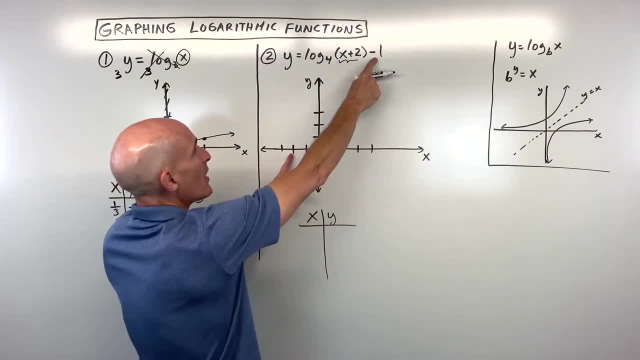 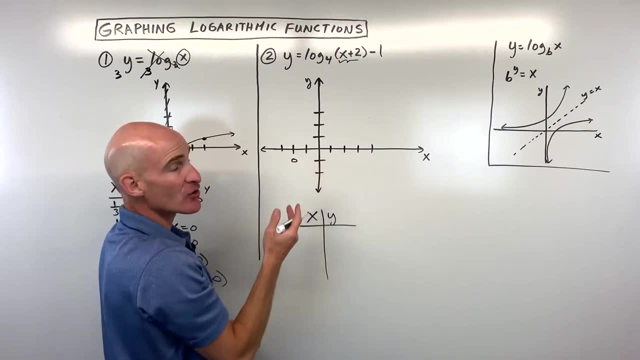 actually going to shift the graph left two, and this minus one. this affects the vertical direction up and down. it's going to shift the graph down one. So you could think of this point right here as like your new starting point, okay, or like your new origin. Then you can. 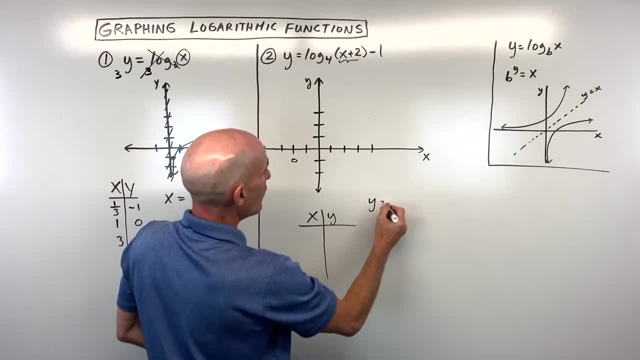 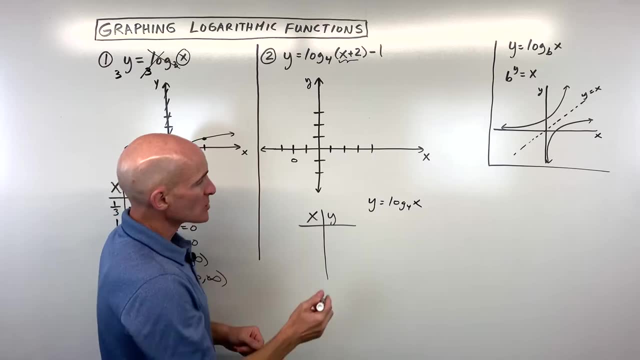 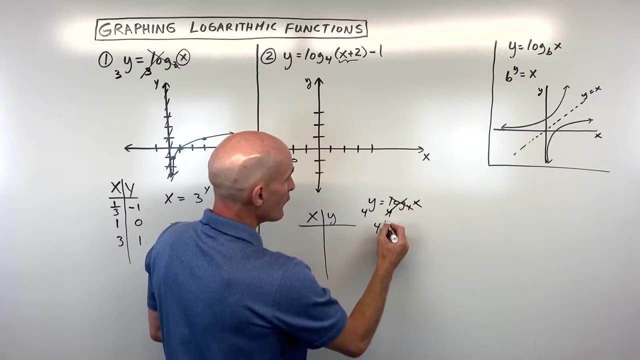 focus in on this parent function, this basic function. y equals log base four of x graph. that, but from the shifted origin. So that's one way to do it. So let's, let's talk about that. So if we exponentiate both sides using this base four, these are inverses of one another. four to the y power. 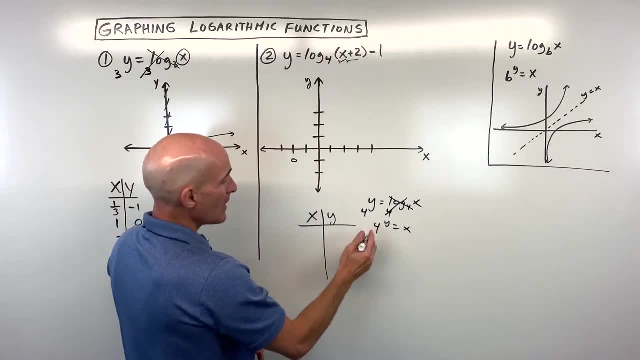 is equal to x. that's just rewritten in exponential form. Plug in some easy numbers. I usually put in negative one zero and one, just some small numbers. Four to the first is four, but in negative you take the reciprocal. So this is one fourth. Four to the zero is one, because anything to the zero power is. 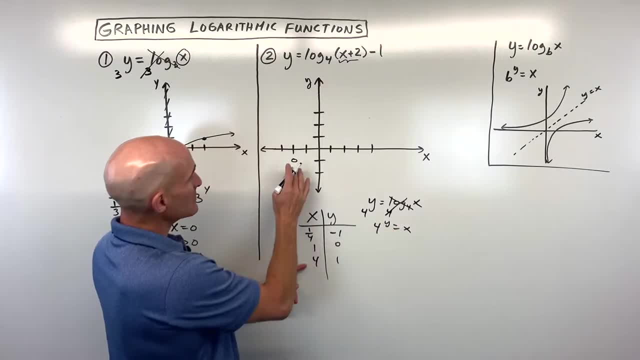 one and then four to. the first is four. I'm going to plot these points from here, So what I can do is I can go right one, fourth, down one. right one up zero. right four, one, two, three, four up one, And you can see this graph is going to look something like: 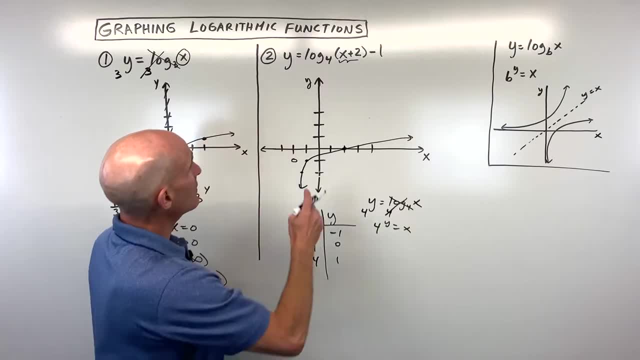 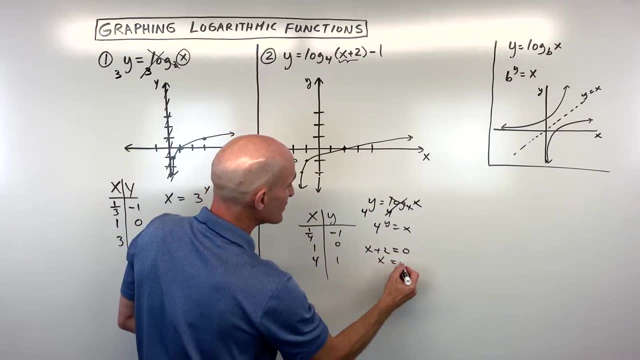 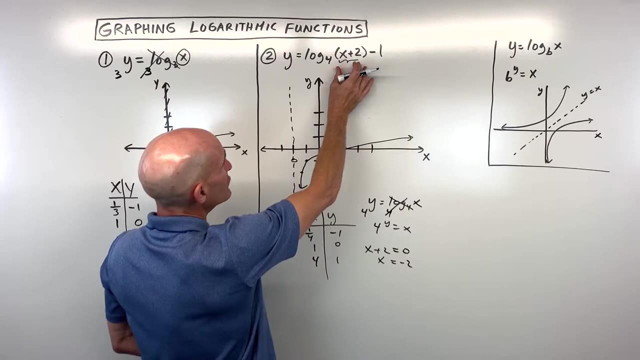 this, Now the domain. remember how we said: if you set this equal to zero, you can find your domain whatever is grouped with the x here. So x plus two equals zero. subtract two x equals negative. two gives you your vertical asymptote, But if you want to find the domain, you'd make this: 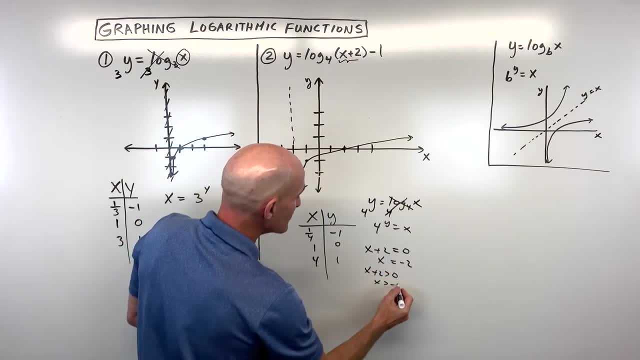 a an inequality: x plus two is greater than zero. x has to be greater than negative two. Or if you're in pre-calculus and you're learning the interval notation, you can say from negative two to infinity and then the range is all real numbers. Okay, it goes down and up forever and ever. Or you could 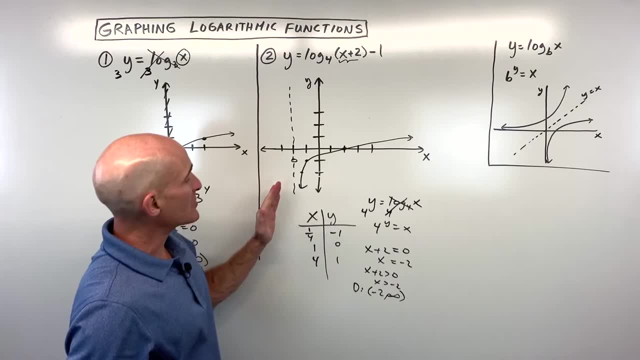 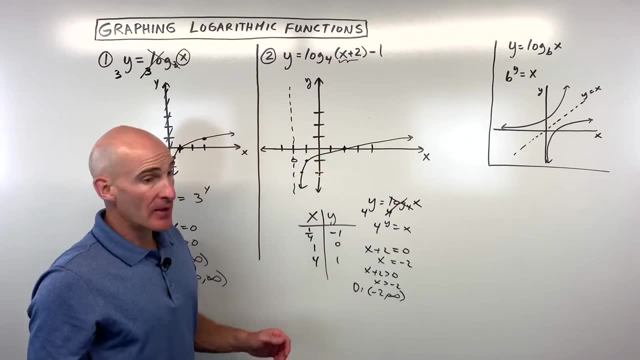 say negative infinity to positive infinity. So that's one option. Another option okay is you could set up your table Okay, just with y equals log base four of x, and then apply the transformations to the table. So you could say: hmm plus two, that's going to shift the graph left two. I. 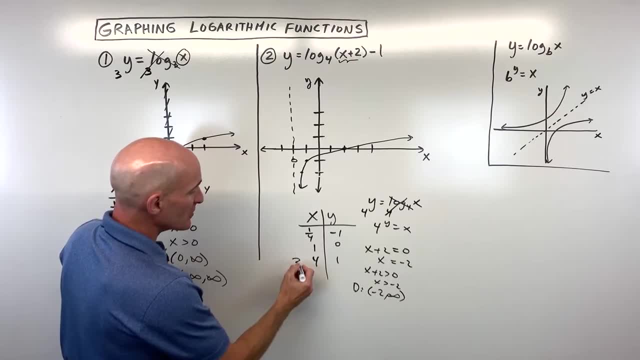 can subtract two from all these y values, So this would be two. this would be negative one, this would be negative one. and three-fourths Cross out the old x values. The minus one shifts it down one. That means you're subtracting one from. 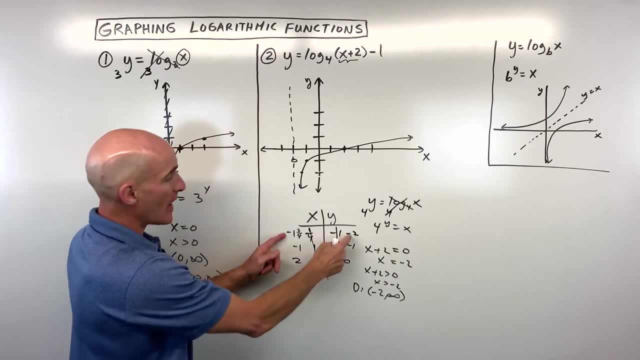 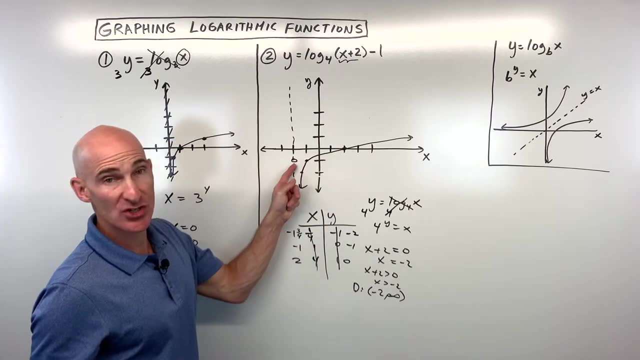 all of the y values Cross out the old ones. Now you can just plot these points from the original origin. Okay, so that's another way to do it, using the table, or you can use a shifted origin. Another option for you: those ones kind of go together. The other option for you is just to 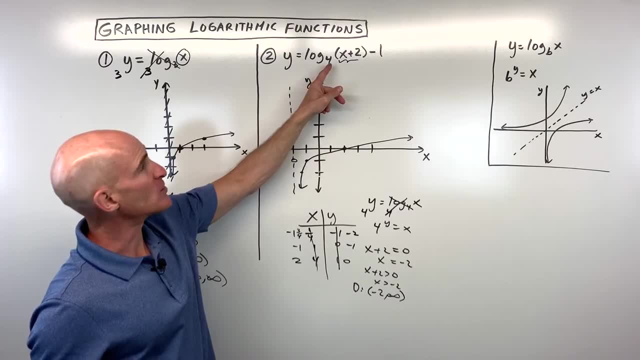 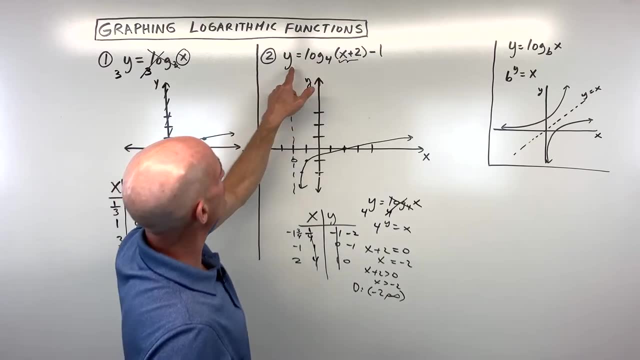 rewrite this in exponential form. So what we're going to do is we're going to try to get this x by two. So what we're going to do is we're going to add one to both sides, So that's going to be y plus. 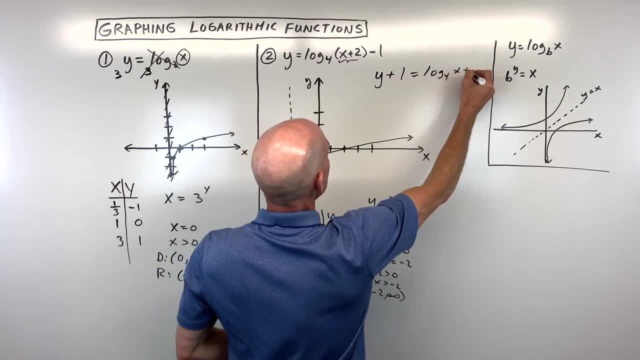 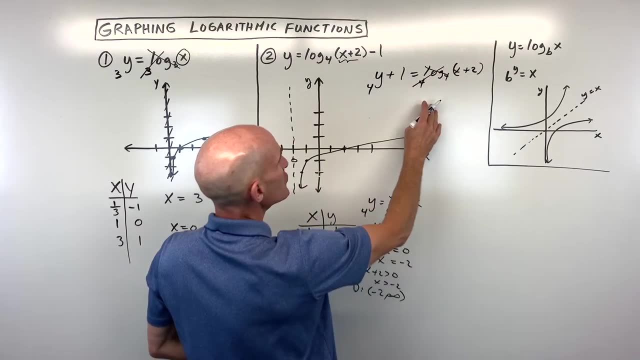 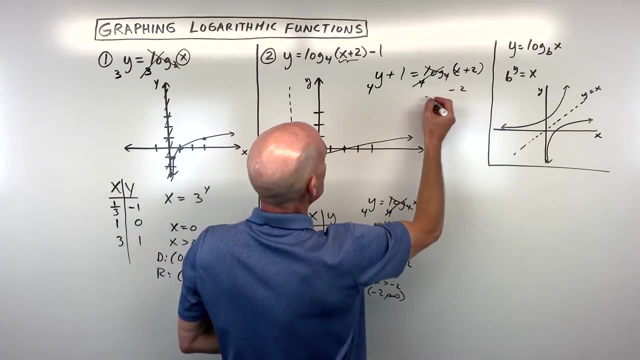 one equals log base four of x plus two. Then we're going to exponentiate both sides using base four. So those are inverses, They undo each other, kind of like adding and subtracting or multiplying and dividing or squaring and square rooting, And then we can subtract two from both sides. 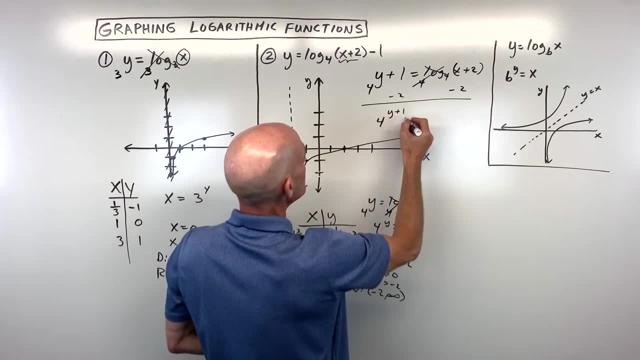 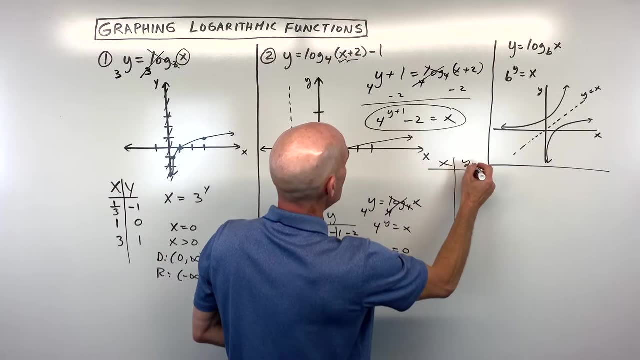 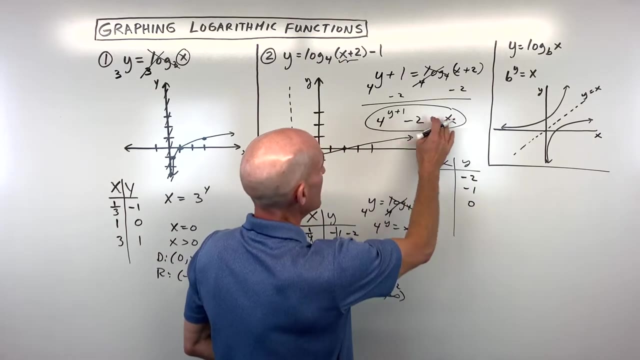 And now what do we have? We have four to the y plus one power. minus two equals x. Now this equation: we can make a table and pick some values for y. So you might want to pick, like, let's just say negative two, negative one and zero. Plug that in, get your x values and 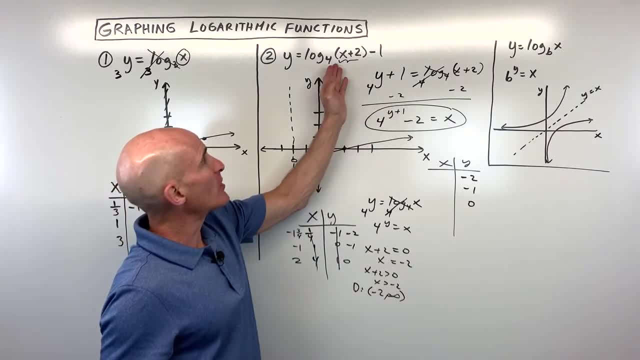 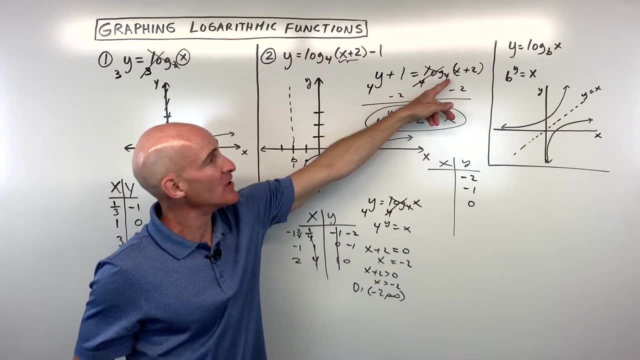 you can graph it like that. So all we did was we got rid of the log, okay, by exponentiating, but we're trying to get this x by itself here. So we're just trying to solve for x by working from the outside in, And now that you're familiar with the exponential notation, we can just plug in. 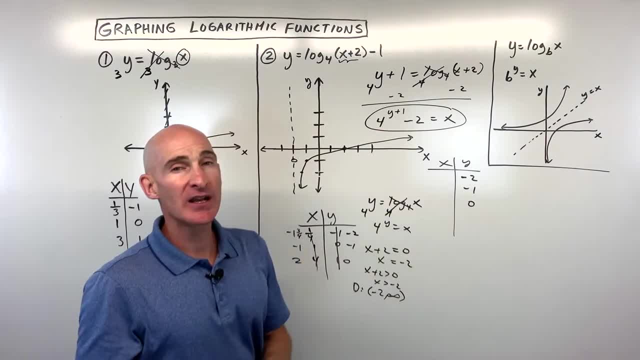 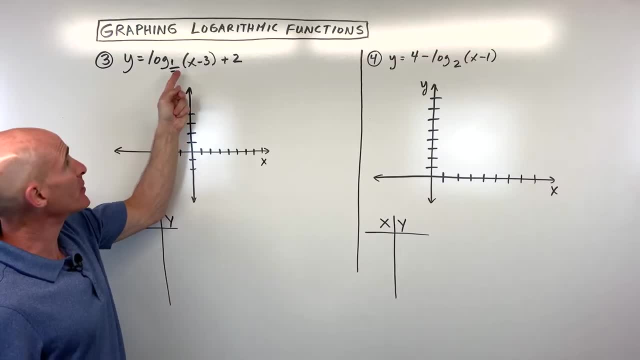 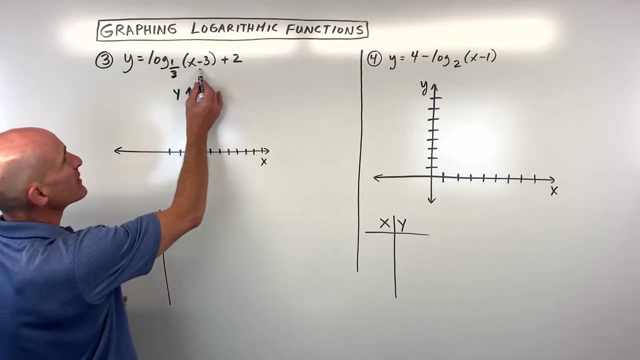 and solve for x. So a couple different options. Let's look at a few more examples. Okay, let's take a look at example number three. now We have y equals log base, one third of x minus three plus two. So let's look at a couple different options here. So this one: we wanted a graph We could think of. 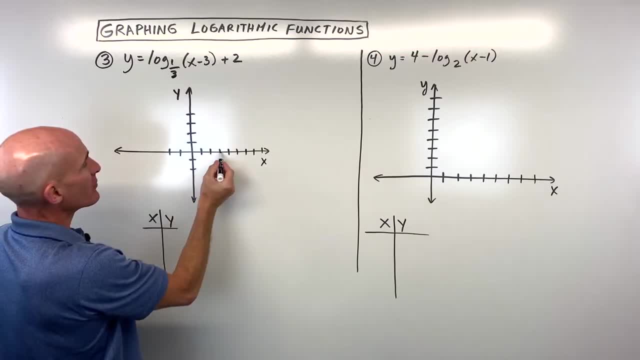 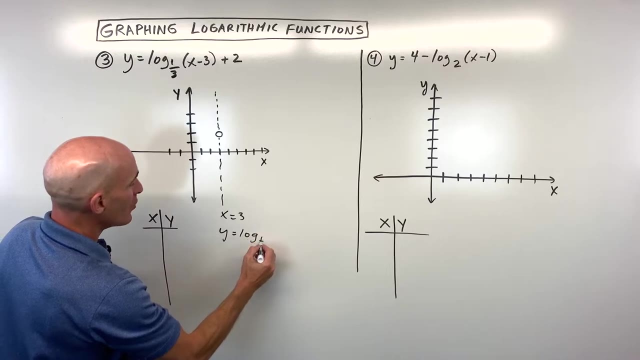 shifting this graph: right three and up two. So you write three up two. You can think of this as your new origin. You could draw your vertical asymptote right through here. That's the line x equals three. You can focus in on the parent function, which is y equals log base: one third of x. Now, what I like to. 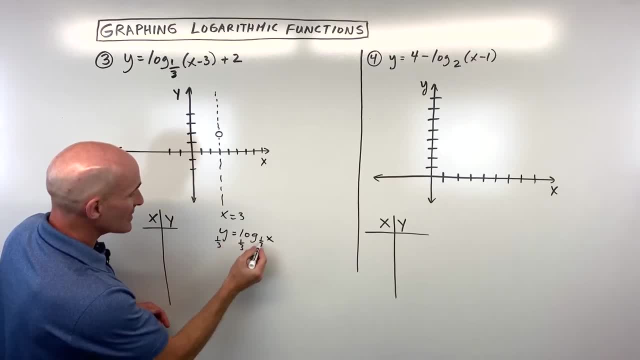 do is I like to exponentiate or raise both sides using the same base- one third, And what that does is that writes this in exponential form. So what I'll do is I'll plot some values for y Negative, one zero and one- One third to the negative. one is three because the negative you take the reciprocal. 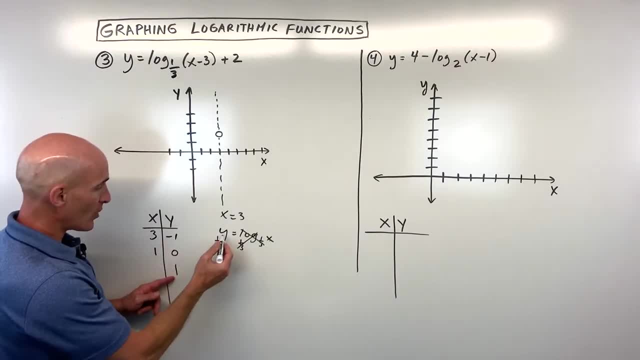 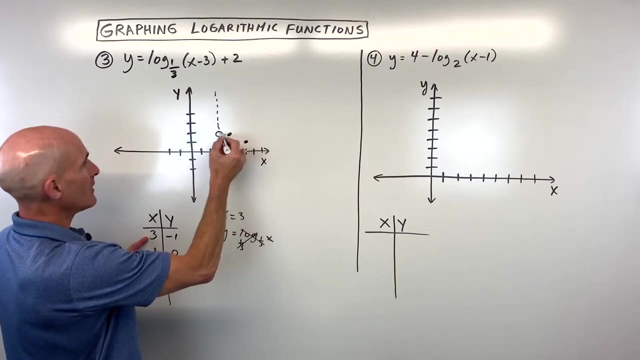 One third to the zero is one. Anything to the zero power is always one. And then one third to the first is itself one third. What we're going to do is we're going to plot these points from this new origin, So we're going to go right, three down one, Right, one up zero, And then right. 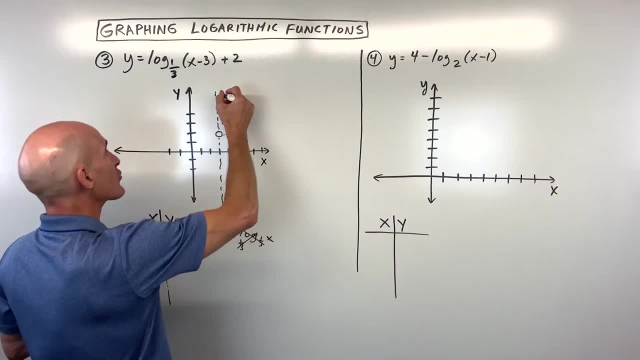 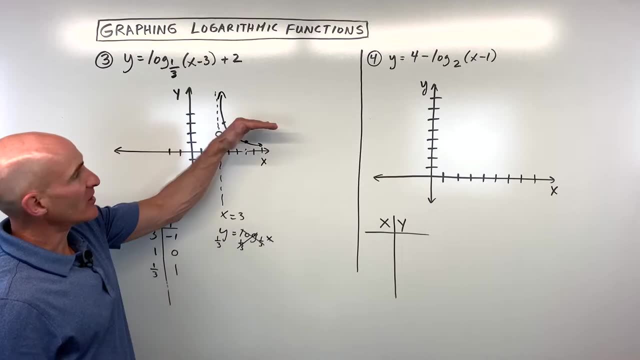 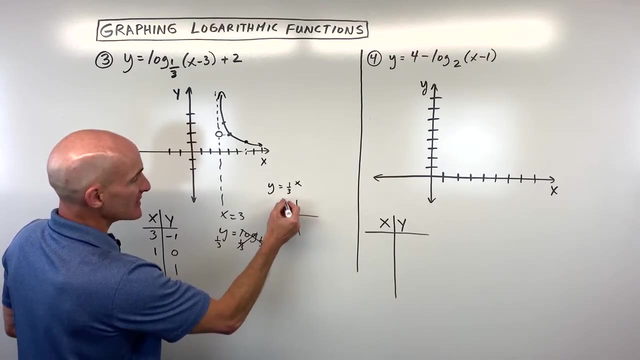 one, third up one, And so your graph looks something like this. Okay, and you might be saying: well, Mario, I thought the log graphs look like this, right. Well, if you think about graphing, y equals the x, See, this is an exponential decay function. When that base is between zero and one, it's going. 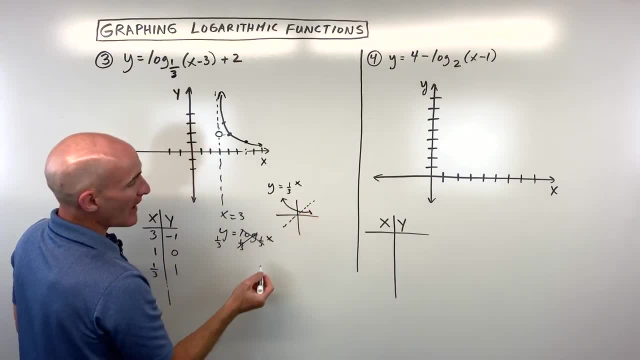 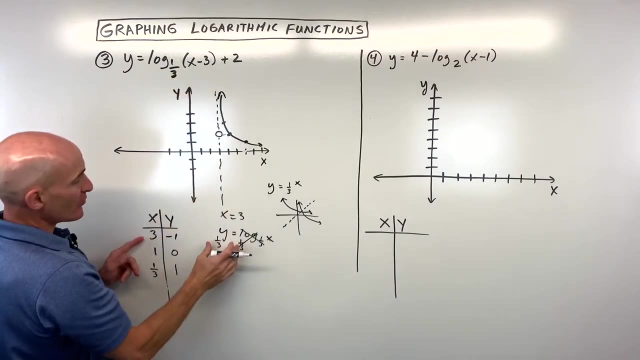 to go down to the right And then, if you reflect it over the line, y equals x, you're going to graph, get a graph that looks something like this: Okay, and so that's why that graph looks like that. Now, another way to do this problem is you can take your parent function, like we just did right here. 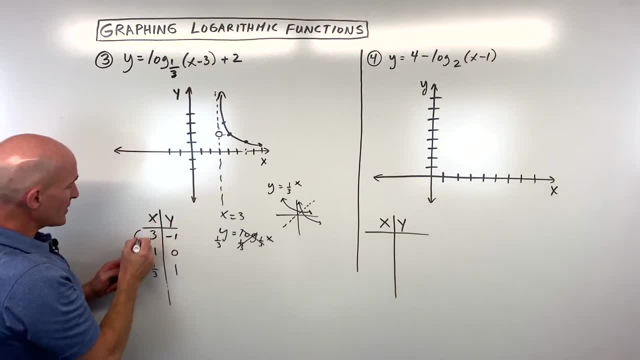 And then, once you have your table, you could add three to all the x coordinates, So that'd be like four and three and one third, And then the plus two shifts everything up to. So if you add two to all of the y coordinates, you could plot these points, But you'd plot them from the original. 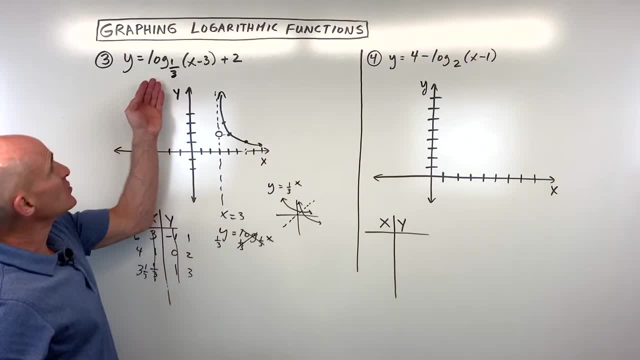 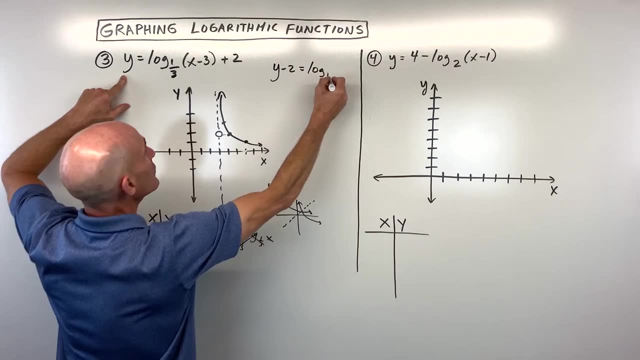 origin: zero, zero. And then the other option is: what you can do is you can solve for x. So what I would do is I would subtract two from both sides of this equation, So it'd be y minus two equals log base one third of x minus three, And then I would exponentiate both sides. 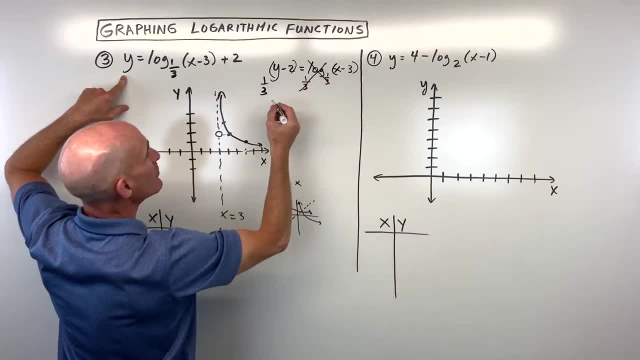 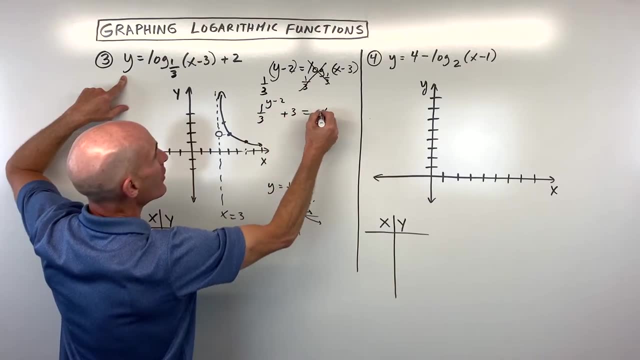 Okay, that way these are inverses, they undo one another. And then I would add three to both sides of this equation. So you're going to get one third y to the y minus two. power plus three more equals x. And then what you can do is make a table. just plug in some values for y, get your x coordinates. 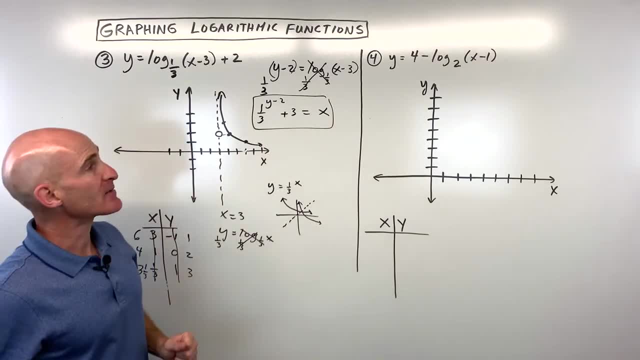 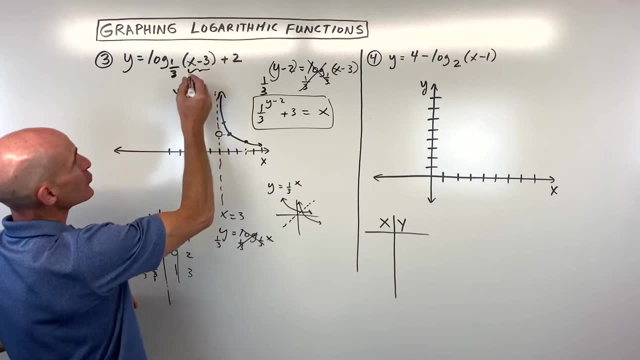 and then plot from the original origin. So you have a few different options with these problems, whichever way you like to approach it. Now, as far as the domain, see whatever is in the parentheses here- a group of the x. this has to be greater than zero. 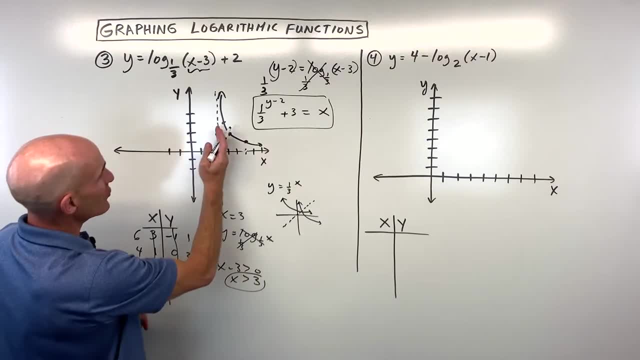 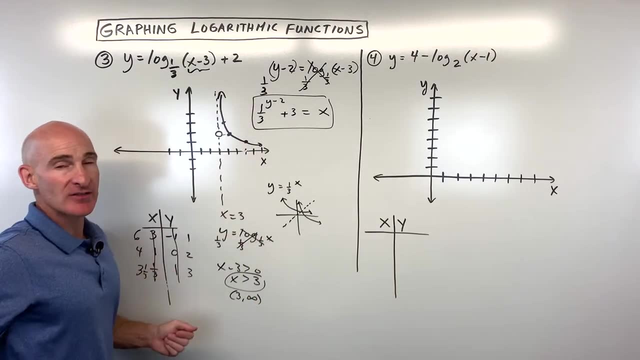 So if I solve that inequality, add three to both sides, x has to be greater than three, Or you could say an interval notation from three to infinity, And then the range for these log graphs is always going to be all real numbers. Okay, let's take a look at example number four Now. 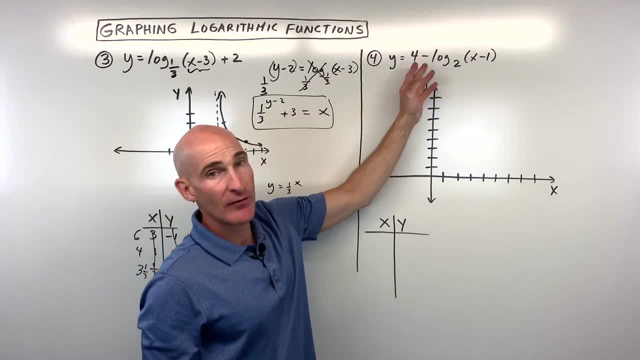 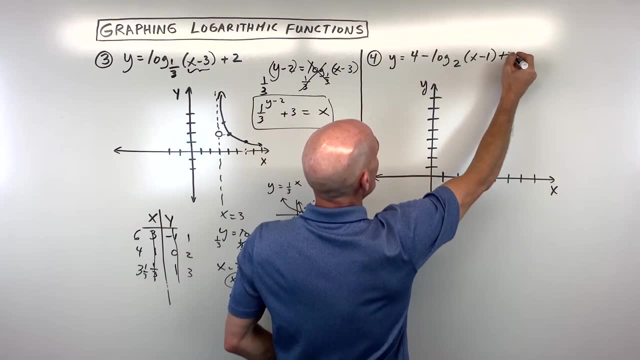 this one is a little bit more challenging, just in the sense of the way that it's written. So you see this four right here. Watch carefully. what I'm going to do is, since this is a positive four, I'm going to put the four over here and I'm just going to subtract the four there. 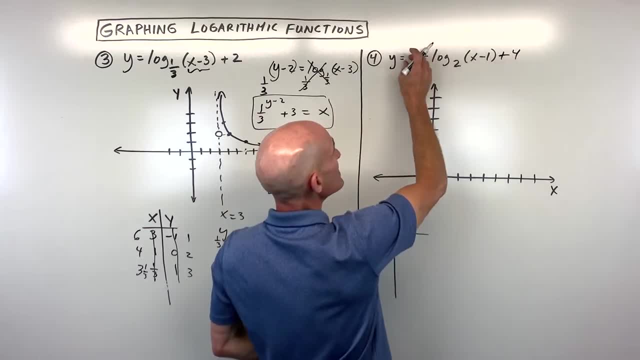 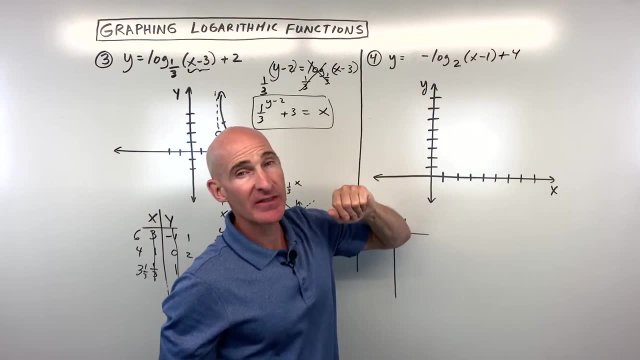 So I'm not really doing anything to both sides of the equation, I'm just putting the four over here instead of in front, Just to kind of rewrite it a little bit. Now this one: we have a negative in front of the log. What do you think that negative does to the graph? Well, it's going to reflect it over the x-axis. 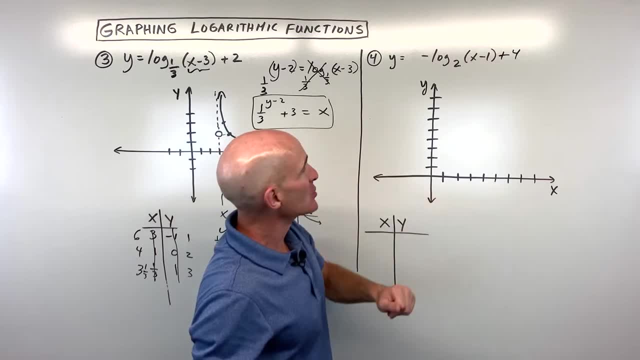 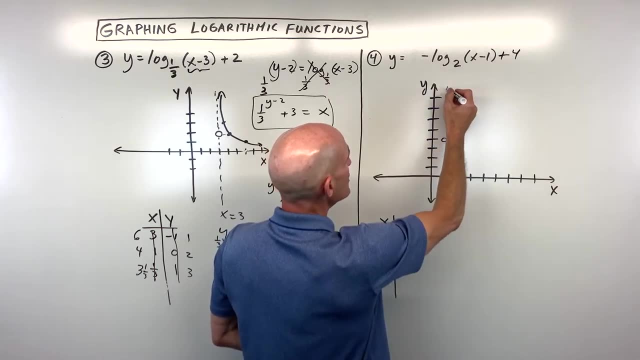 It's going to make all the y values the opposite sign. So what you can do, you can still do like we were doing before. You can say this is going to shift right one up four. You can think of that as like your new origin. Here's your vertical asymptote. This is the line x equals one. Remember vertical lines are x equals one. 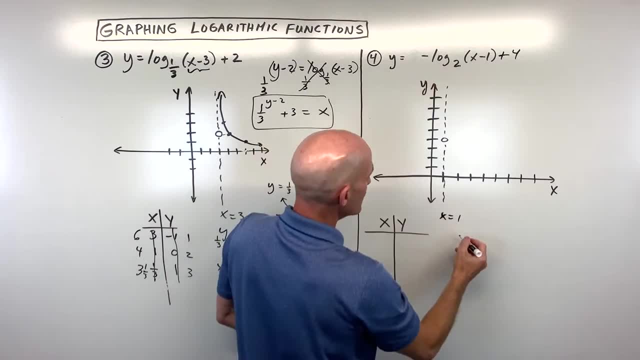 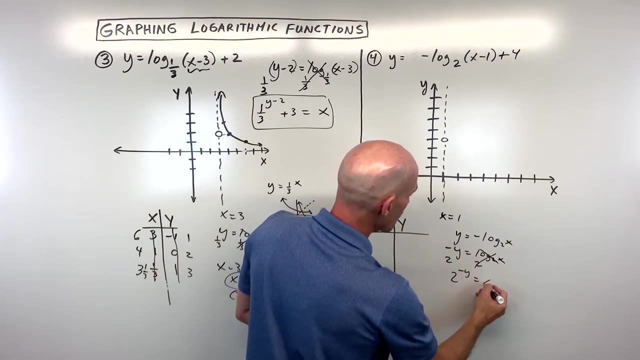 And then what we'll do is we'll focus on this parent function here. y equals negative log base two of x. Now you might want to multiply both sides by negative one And then when you exponentiate both sides, you can see this is two to the negative. y power equals x. 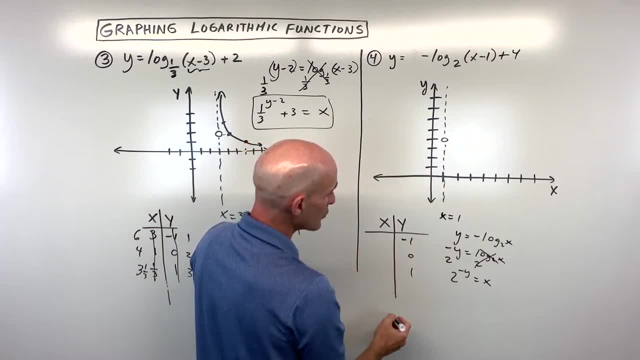 So we'll go ahead and plot some values for y, like negative one, zero one. A negative times. a negative gives you positive one. Two to the first is two, Two to the zero power is one, And two to the negative one is going to give you one half. 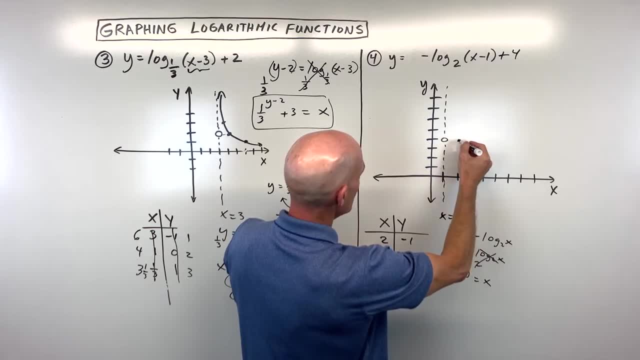 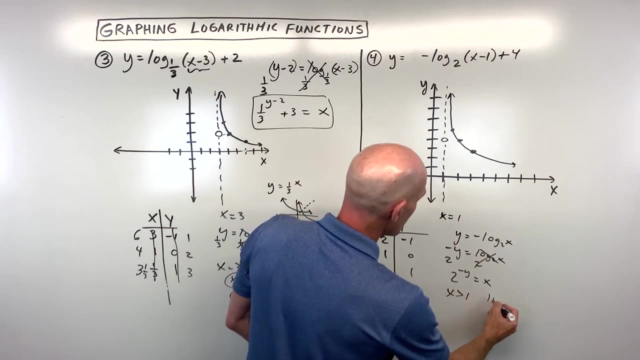 Plotting from here. now. write down, one would be right about here. Write 1: 0 would be right about here. Write a half up. one would be right about here, And you can see your graph is looking something like that Domain would be: x is greater than one, or you could say from one to infinity. if you're using the. 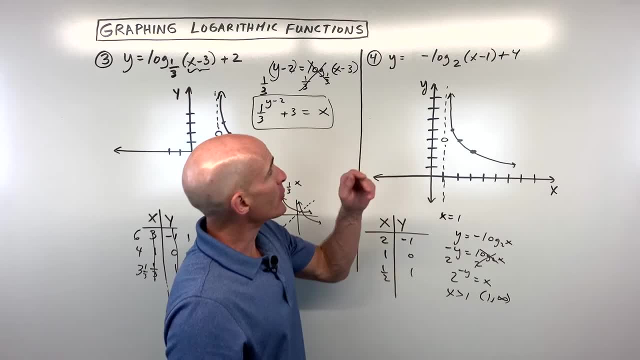 interval notation Ranges is all real numbers. The other option you could do is you could think about Salvador to be x to 1.. The other option you could do is you could think about Salvador to be x to 1.. And that's what a zona value is a Taylor, because if you put the capital Filipino and inverse to it, what you get r of y is 5b. 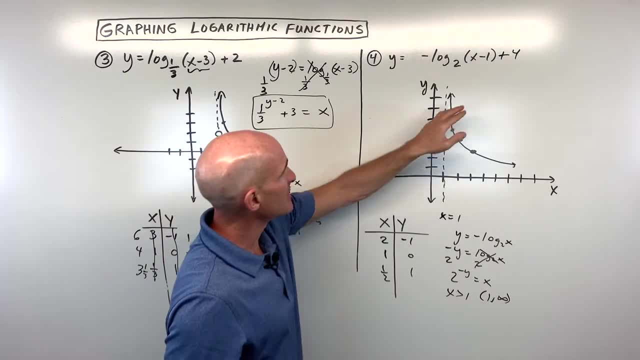 It's not always low and sometimes it, whereas either c is 0 and another č, but that's the top one, so it's still going to be fine. Another option you could do is you could think about the dimension of your model, is you could think about the transformations You could say, starting from the inside, working your 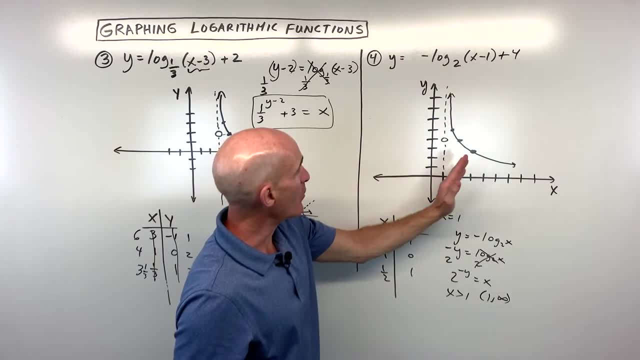 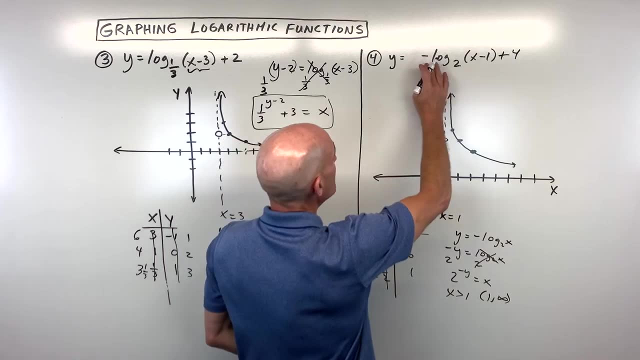 way out. you could say: minus one that's going to shift the graph right, one which is going to add one to our x values. so three, two, one and a half, and then this negative is going to make all the y values the opposite. so this would become a positive one, zero, negative one, and then the plus. 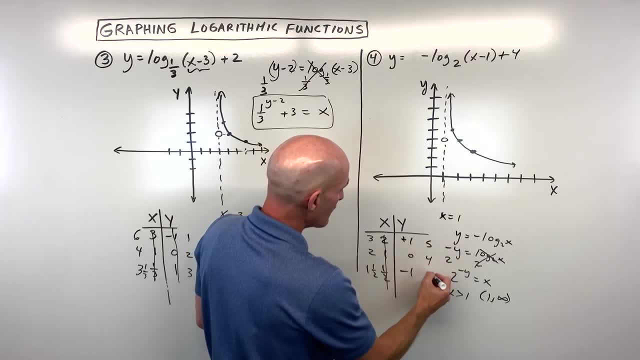 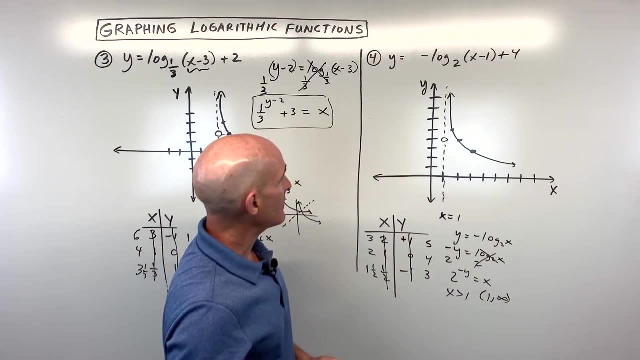 four shifts everything up four. so adding four to the y's is going to be five, four and three, and then you can plot these points from the original origin. and the other option is you could try to solve for x. so what you could do is you could subtract four from both sides, so y minus four. 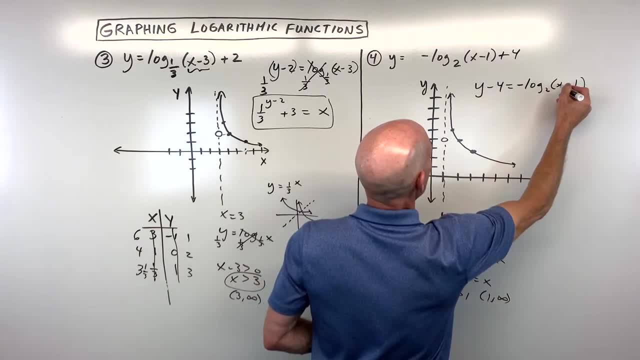 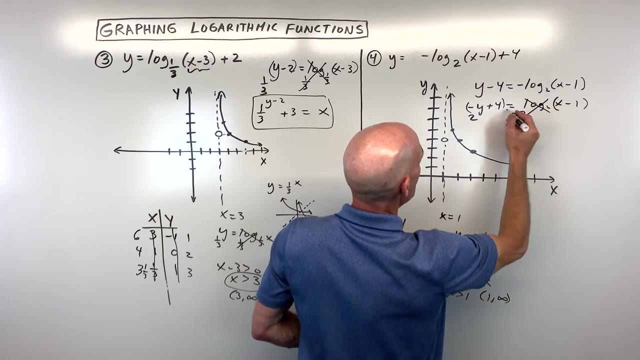 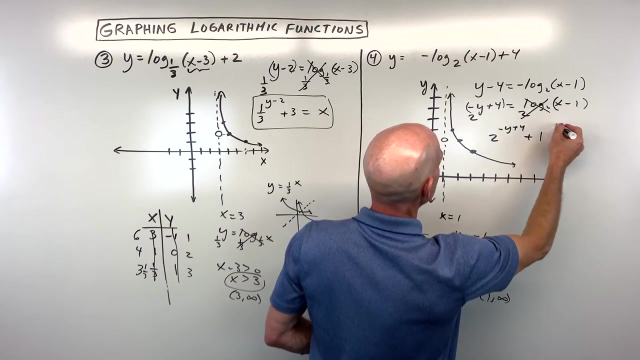 equals negative log base two of x minus one. multiply both sides by negative one, so that would give you negative y plus four equals log base two of x minus one. exponentiate both sides using base two- these are inverses- and then add one to both sides so you'd have two to the negative y plus four plus one equals x. and then now you can just 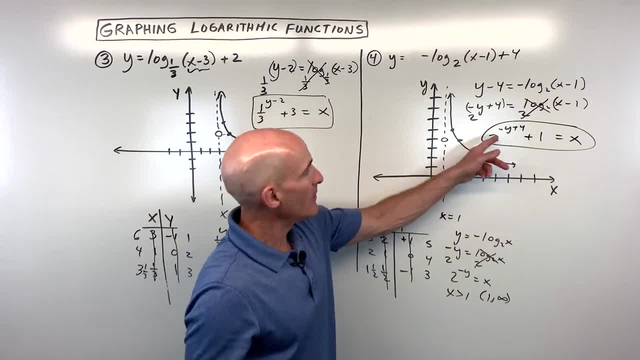 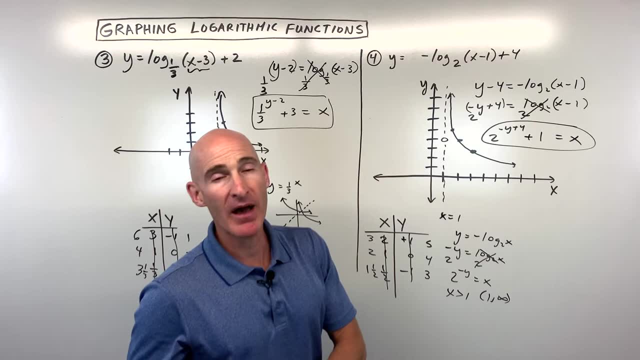 use this entire equation, plotting from the original origin. pick some values for y, get your x coordinates and plot. so whichever method you like, the best you know, go with that method. let's look at two more examples. see if you can do these on your own. okay, pause the video. see what you can. 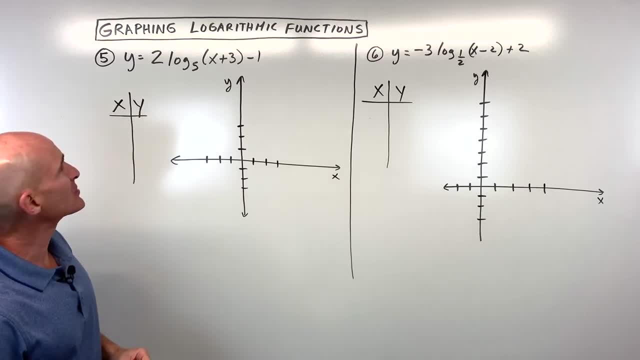 do for number five and number six. now for number five, if i was going to approach this problem again, remember there's different ways to do it, but what i would probably do on this one is look at the transformations. so i would start with the parent function, which is y equals log base five of x, and then i would exponentiate both sides using base five. 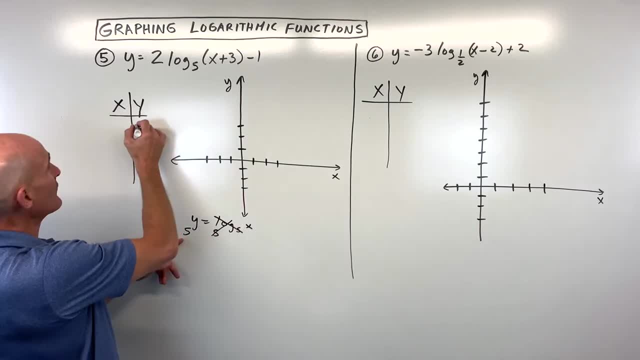 and so this is our basic function. five to the y equals x. so if i plug in some small numbers here, five to the negative, one is one. fifth, five to the zero is one and five to the first is five. but then, working from the inside out, the plus three is going to shift the graph left three. 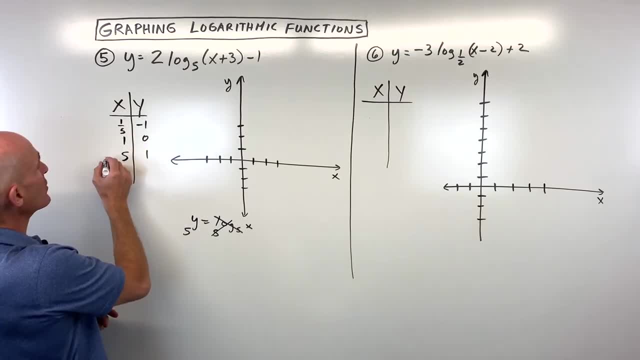 so if i subtract three from all these x coordinates, that's going to give us two, that's going to give us negative one and that's going to give us a negative two and four fifths, and this two here is going to be a vertical stretch by a factor of two, which is going to 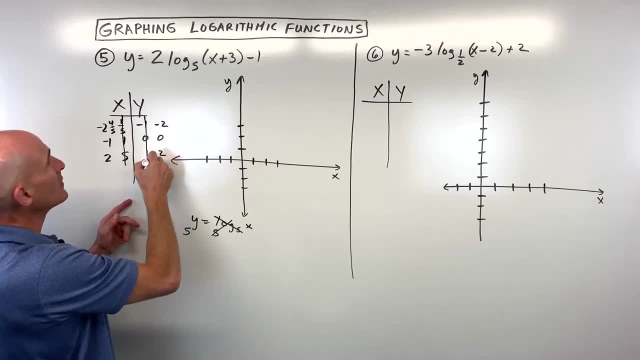 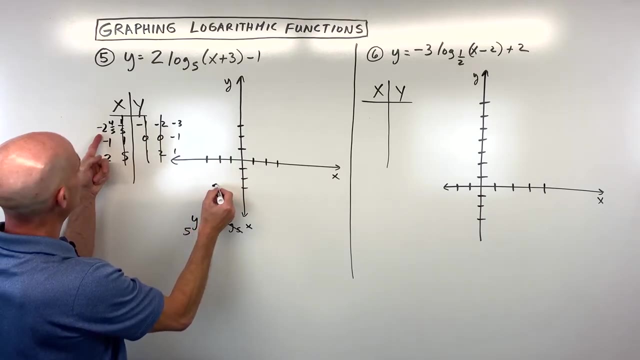 multiply all the y values by two, and then this minus one is going to shift the graph down one, which is going to subtract one from each of these y values. so now you can see- here's some points. we've got two and four, fifths, negative three, which is right about here. negative one, negative one, it's right. 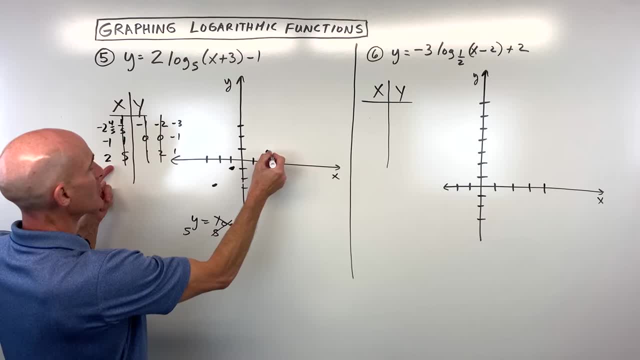 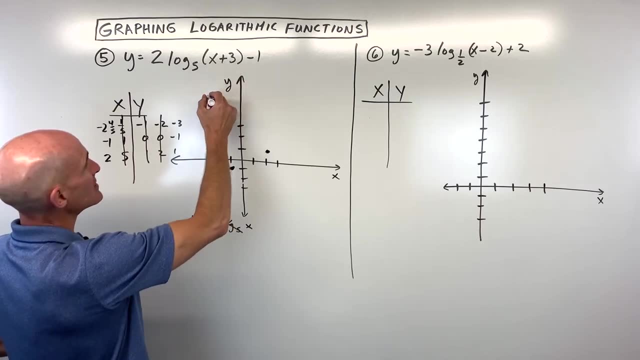 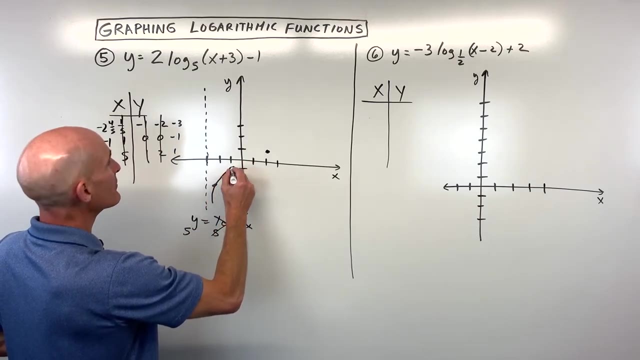 about here and two, one is right about here. okay, so now we can see that our vertical asymptote, if we set this, equal to zero x plus three equals zero x equals negative. three is our vertical asymptote and our graph. this is just a rough sketch, but our graph is going to look something. 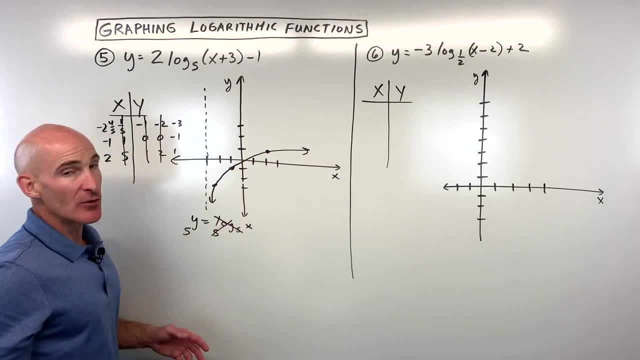 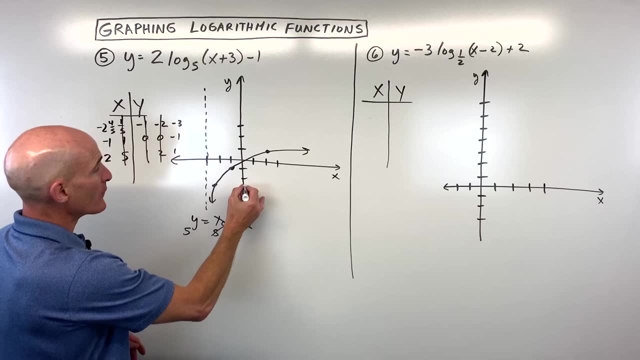 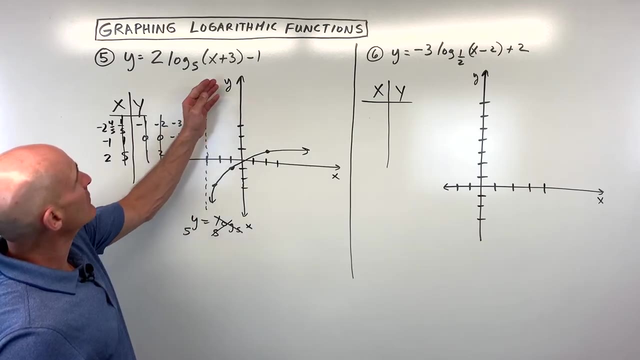 like like this: okay, now you can be a little bit more precise about finding where it crosses the y-axis and the x-axis by setting the opposite variable equal to zero. but for now this is just a sketch. now the other option is: what is to think about solving for x? so we could say: let's add one. 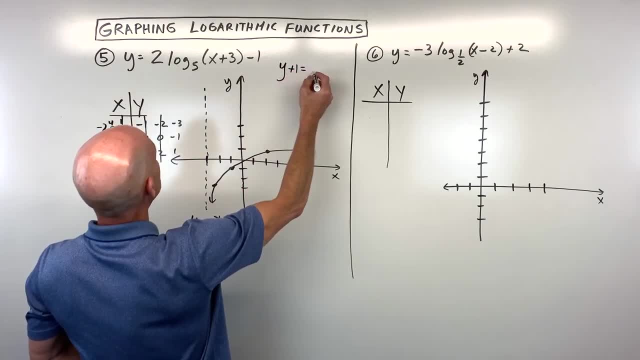 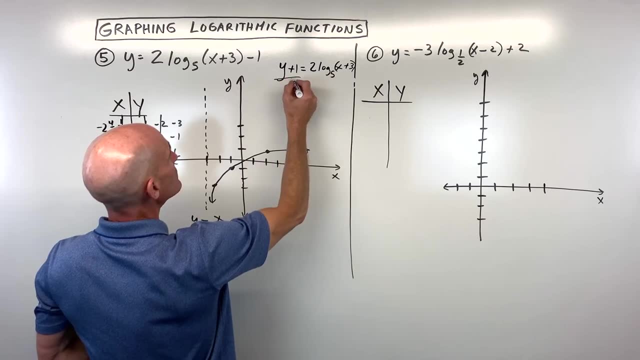 to both sides, so that's going to give us: y plus 1 equals 2. log base 5 of x plus 3. divide both sides by 2 and then exponentiate both sides using base 5, so that's going to give us 5 to the y plus 1 over 2 power equals x plus 3. 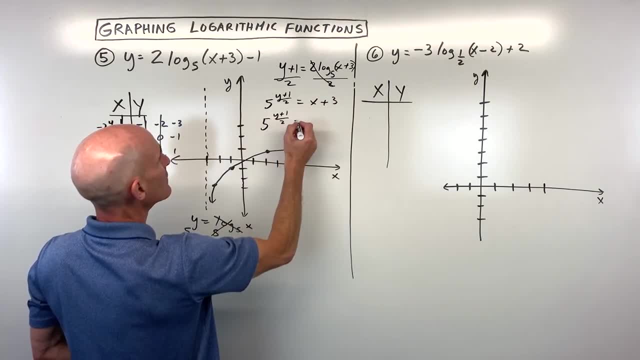 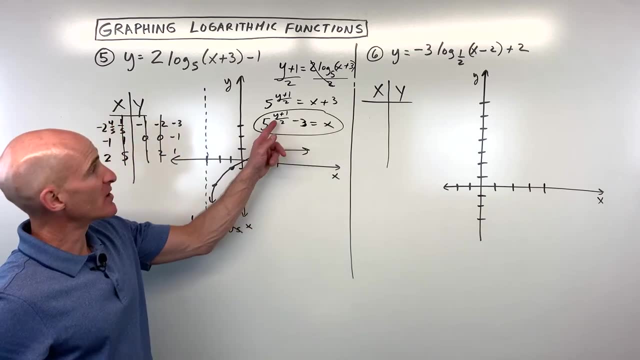 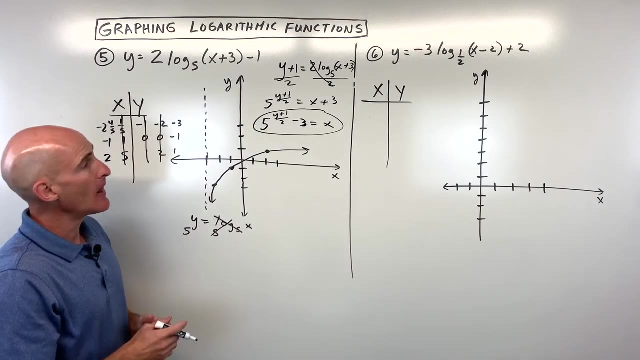 and subtract 3 from both sides equals x. and now you can see we can use this equation: just plug some values in for y and solve for x and you can plot your points like that. so a couple different options, transformations or rewriting, solving for x. let's jump to the last example, number six, here. 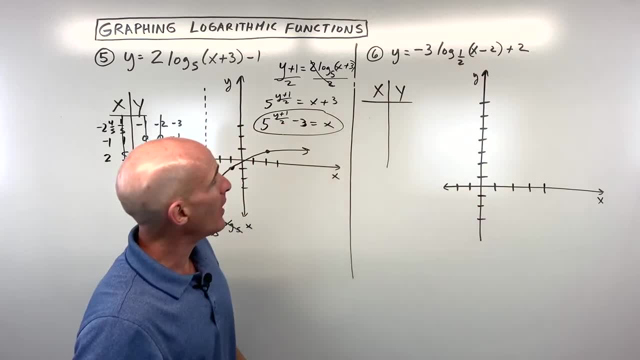 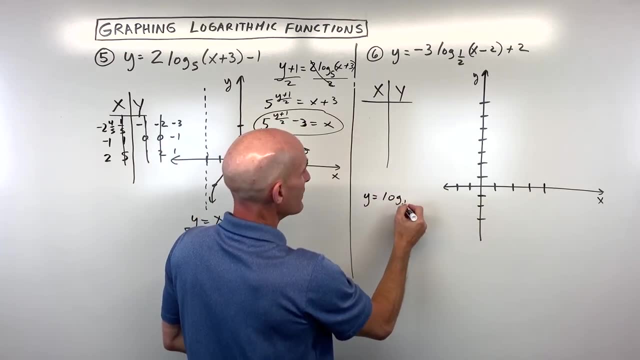 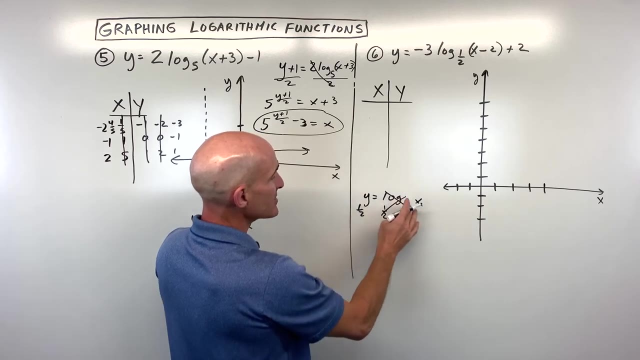 how would you graph this one? well, i'll start off by doing the transformations again. i'd start with the basic parent function, which is: y equals log base one half of x. let's exponentiate both sides by raising both sides using base one half. this is our basic function. if we plug in some values for y. 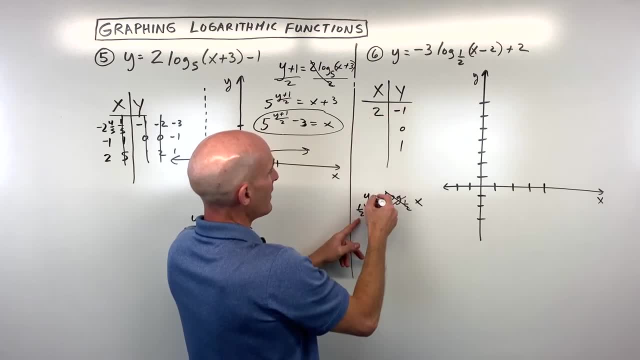 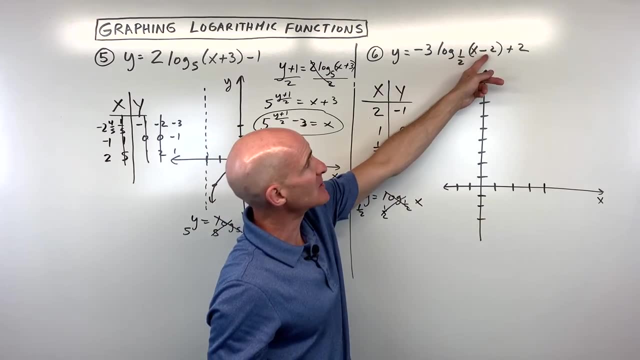 we get two: one half to the zero is one, one half to the first is one half. but then talking about our transformations working from the independent function, we just have to do this, so that's why i'm side out. the minus 2 is going to shift the graph right 2, which is like adding 2 to our 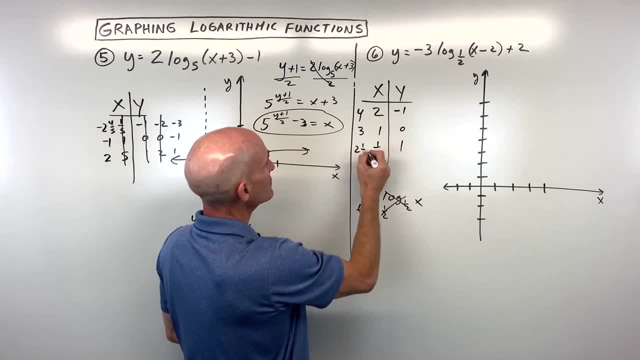 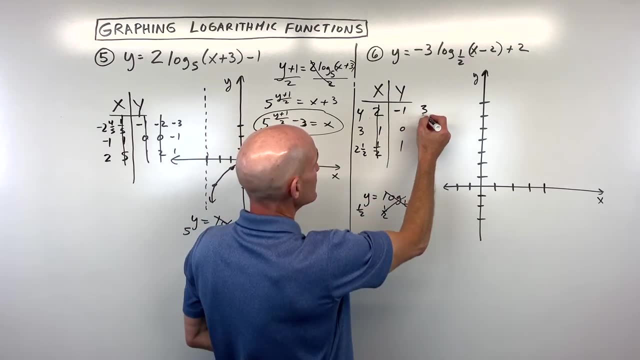 x coordinates. so that would be 4,, 3,, 2 and 1 half. The negative 3 is going to multiply all the y values by negative 3, so this is 3, 0,, negative 3, and then the plus 2 shifts. 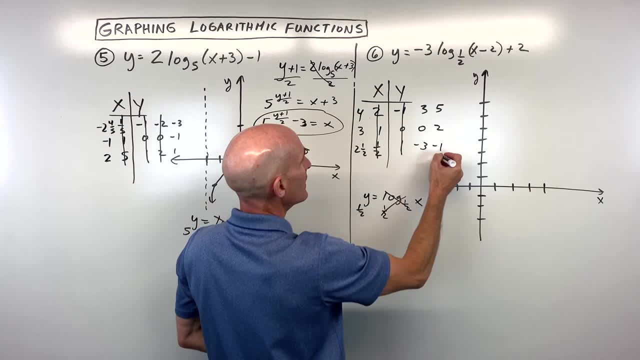 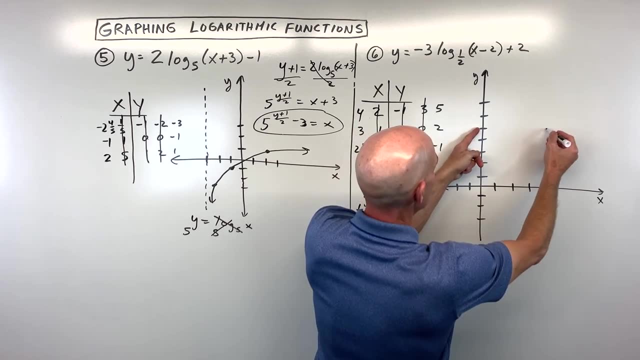 the graph up 2.. That's going to give us 5, 2, and negative 1.. So now we can plot these points: write 4 up, 5,, which is right about here- 3, 2,, which is right about here, and. 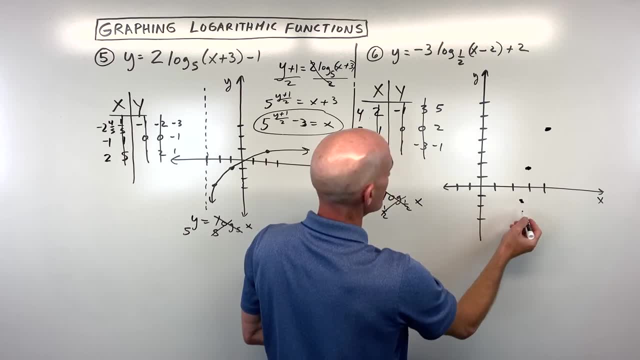 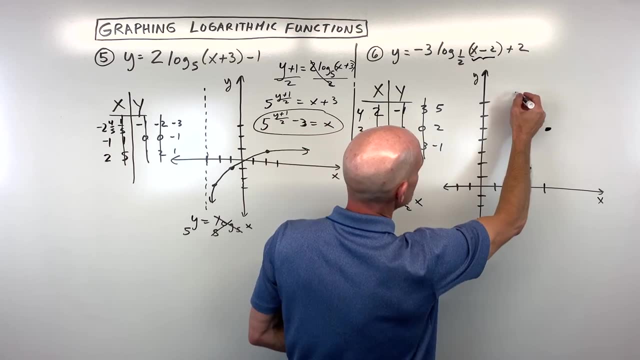 2 and a half negative 1,, which is right about here. As far as the vertical asymptote goes, you can set what's inside the parentheses here equal to 0, and that's going to give you x equals 2, that's our vertical asymptote, and you can make an inequality and make this.